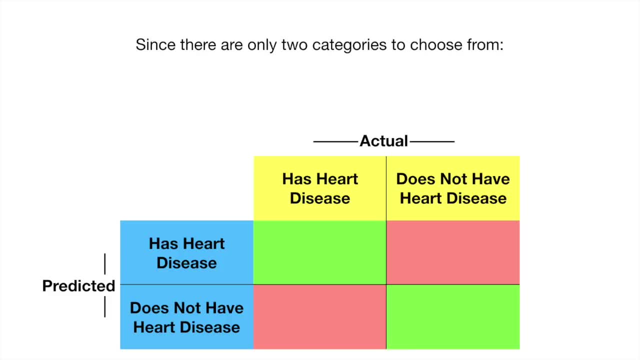 Since there are only two categories to choose from: heart disease or does not have heart disease, then the top left corner contains true positives. These are patients that had heart disease that were correctly identified by the algorithm. The true negatives are in the bottom right-hand corner. 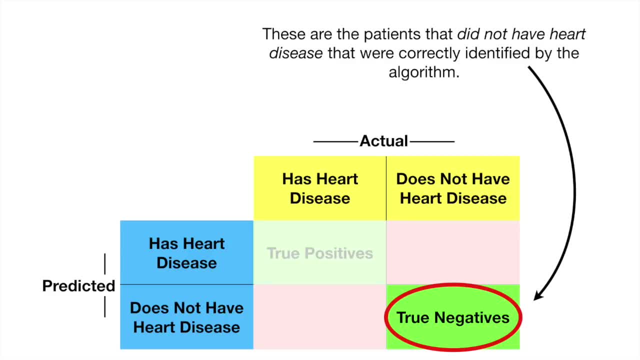 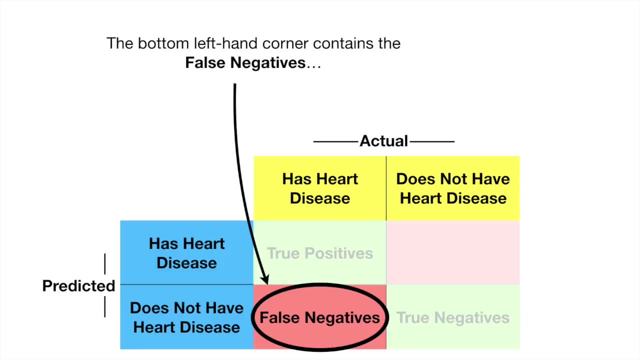 These are patients that did not have heart disease that were correctly identified by the algorithm. The bottom left-hand corner contains false negatives. The true negatives are when a patient has heart disease, but the algorithm said they didn't. Lastly, the top right-hand corner contains false positives. 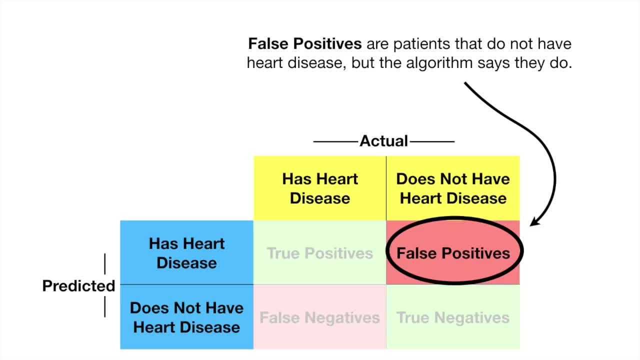 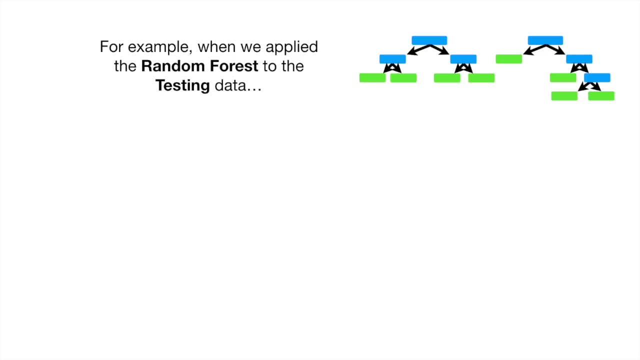 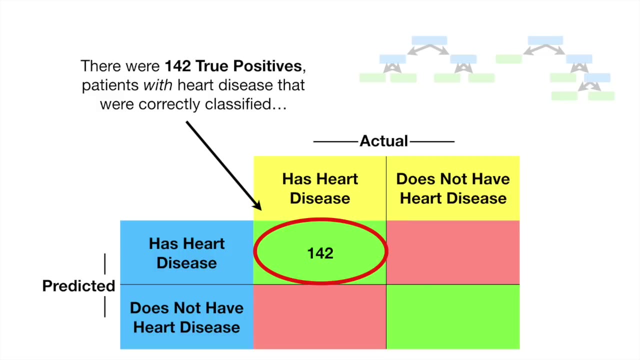 False positives are patients that do not have heart disease but the algorithm says they do. For example, when we applied the random forest to the testing data, there were 142 true positives- patients with heart disease that were correctly classified And 110 true negatives- patients without heart disease- that were correctly classified. 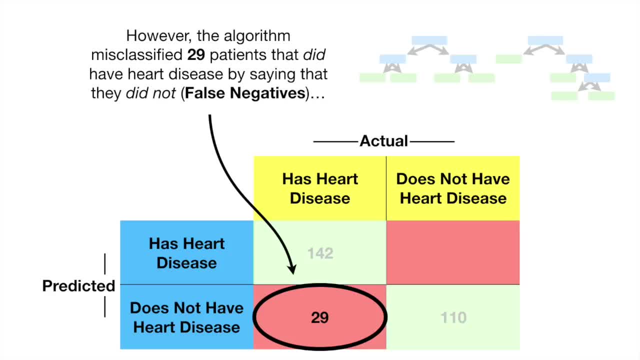 However, the algorithm misclassified 29 patients that did have heart disease by saying they did not. These are false negatives. And the algorithm misclassified 22 patients that did not have heart disease by saying that they did. These are false positives. The numbers along the diagonal, the green boxes: 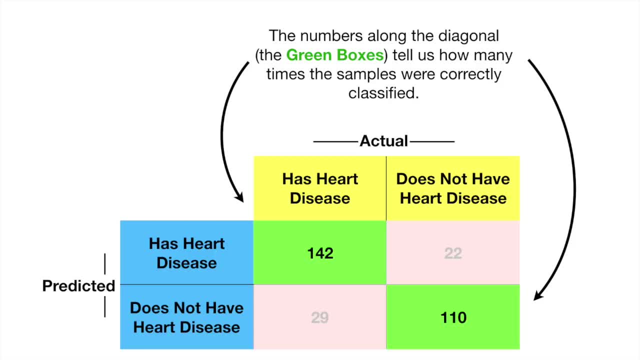 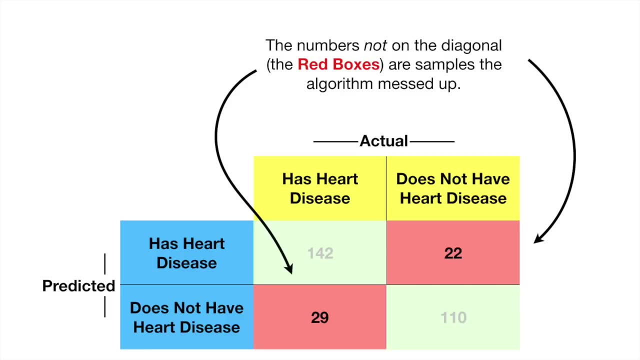 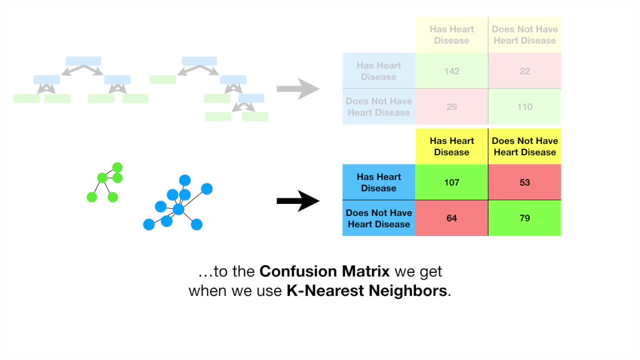 tell us how many times the samples were correctly classified. The numbers not on the diagonal, the red boxes, are samples that the algorithm messed up. Now we can compare the random forest confusion matrix to the confusion matrix we get when we use k-nearest neighbors. 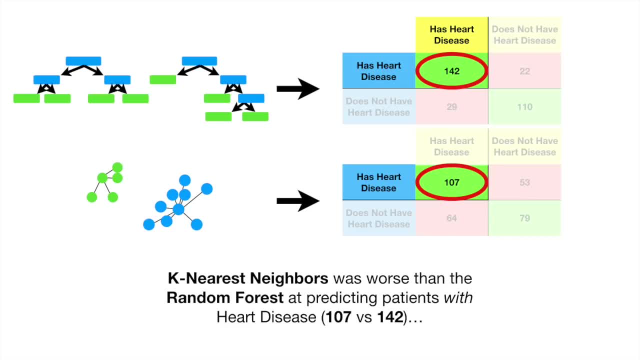 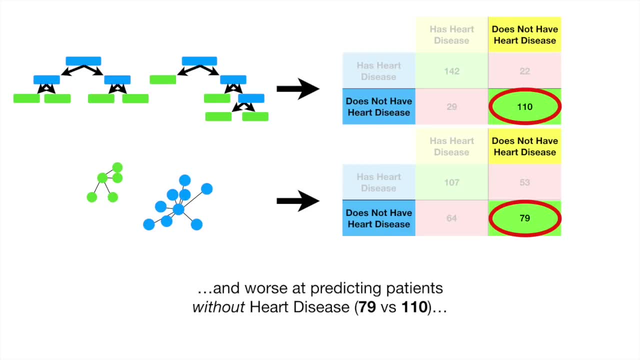 k-nearest neighbors was worse than the random forest at predicting patients with the heart disease- 107 versus 142.. And worse at predicting patients without heart disease: 79 versus 110.. So if we had to choose between using the random forest and k-nearest neighbors, 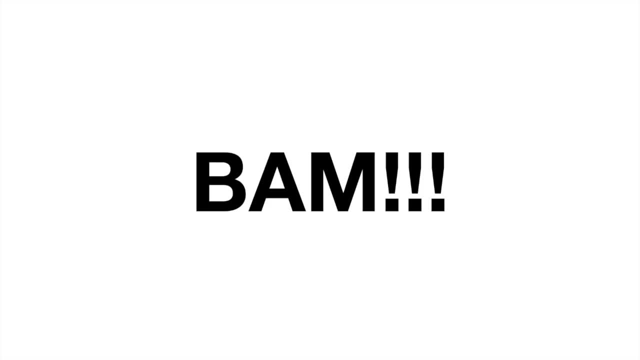 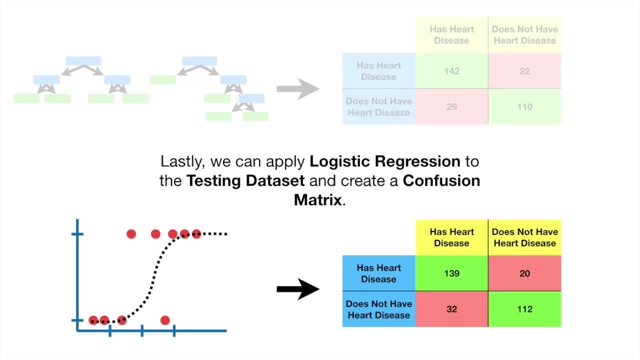 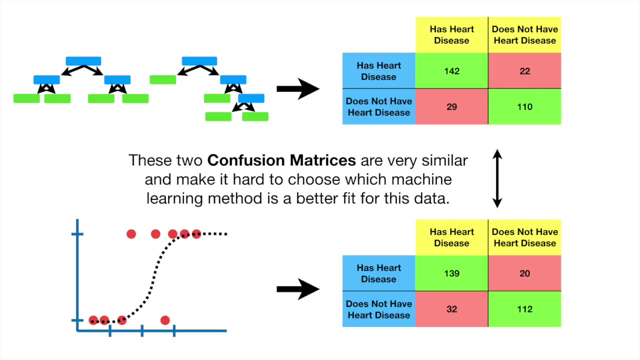 we would choose the random forest Bam. Lastly, we can apply logistic regression to the testing data set and create a confusion matrix. These two confusion matrices are very similar and make it hard to choose which machine learning method is a better fit for this data. 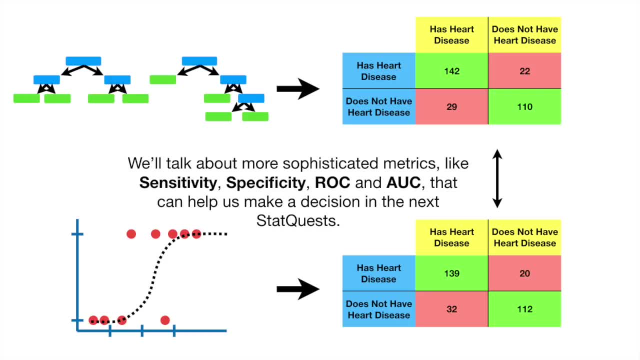 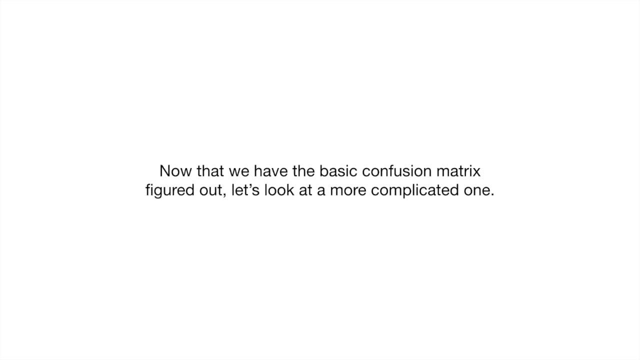 We'll talk about more sophisticated metrics like sensitivity, specificity, ROC and AOC that can help us make a decision in the next stack quests. Now that we have the basic confusion matrix figured out, let's look at a more complicated one. Here's a new data set. 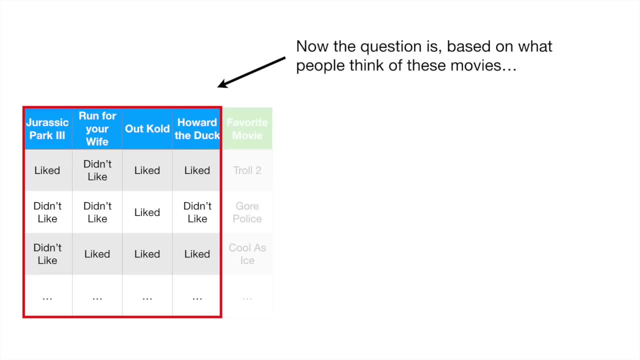 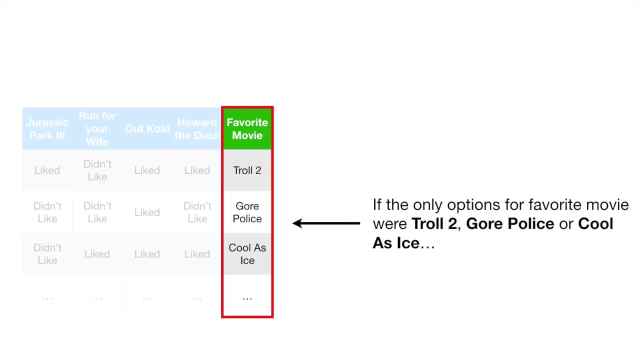 Now the question is based on what people think of these movies: Jurassic Park 3, Run for Your Wife Out, Cold, spelled with a K, and Howard the Duck. can we use a machine learning method to predict their favorite movie If the only options for favorite movie were? 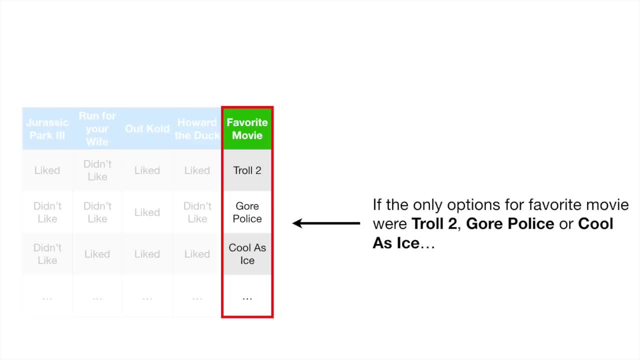 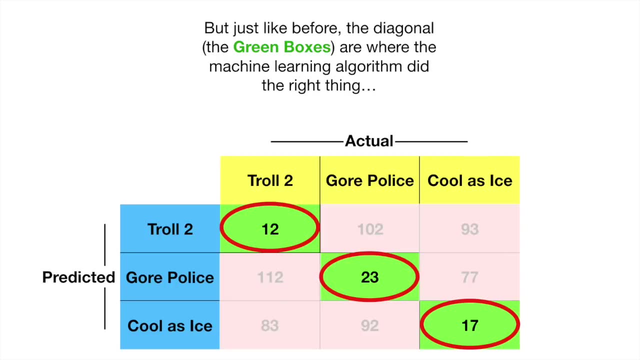 Troll 2, Gore Police or Cool as Ice. then the confusion matrix would have three rows and three columns, But, just like before the diagonal, the green boxes are where the machine learning algorithm did the right thing And everything else is where the algorithm messed up. 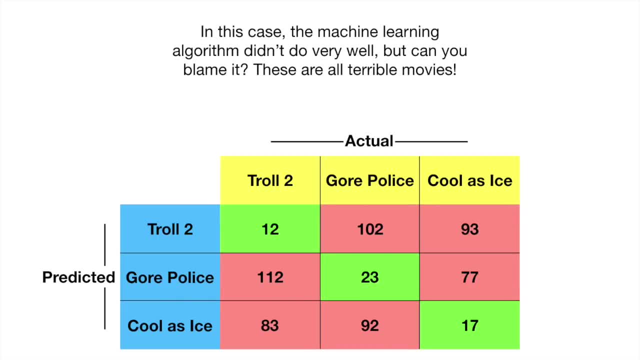 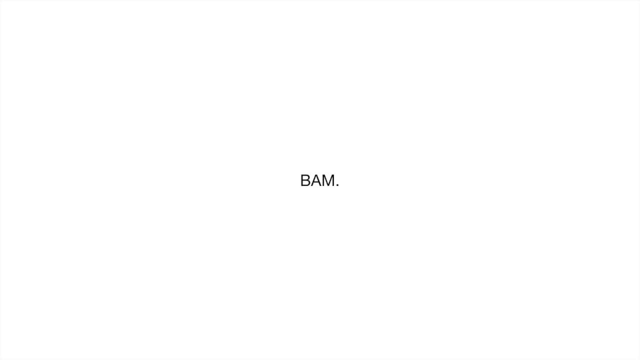 In this case, the machine learning algorithm didn't do very well, But can you blame it? These are all terrible movies, Bam. Ultimately, the size of the confusion matrix is determined by the number of things we want to predict. In the first example. 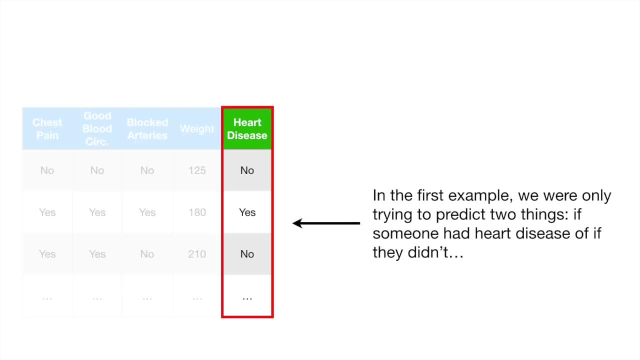 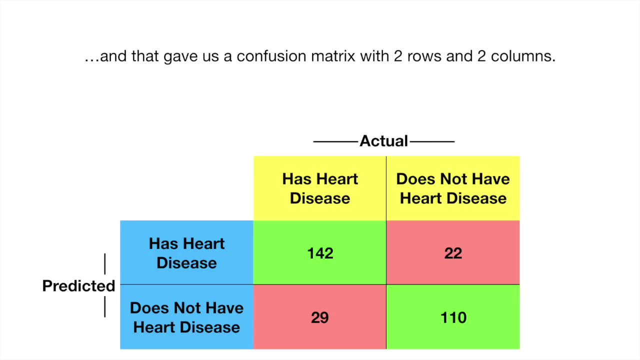 we were only trying to predict two things: if someone had heart disease or if they didn't, And that gave us a confusion matrix with two rows and two columns. In the second example, we had three things to choose from and a confusion matrix. 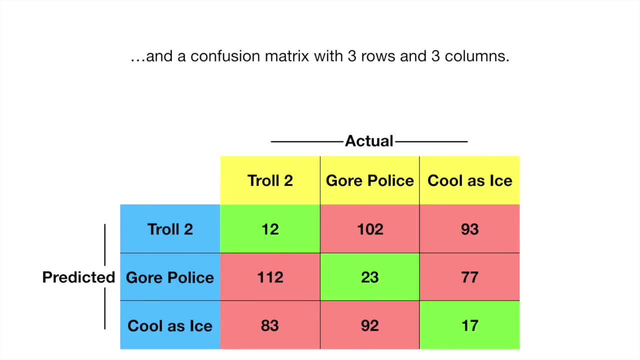 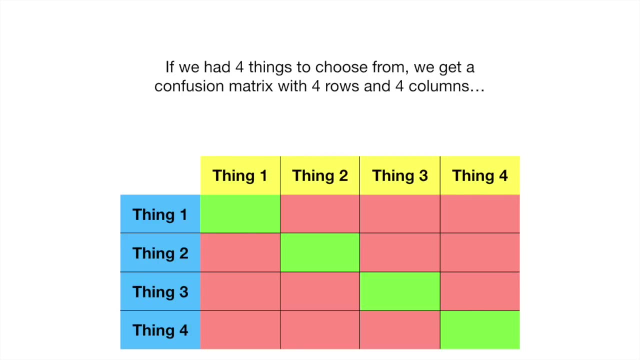 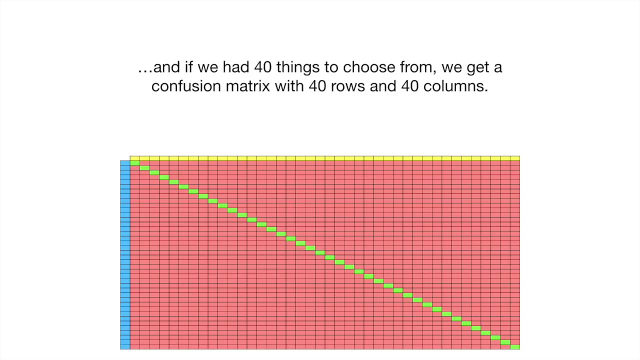 with three rows and three columns. If we had four things to choose from, we get a confusion matrix with four rows and four columns. And if we had forty things to choose from, we get a confusion matrix with forty rows and forty columns- Double bam.